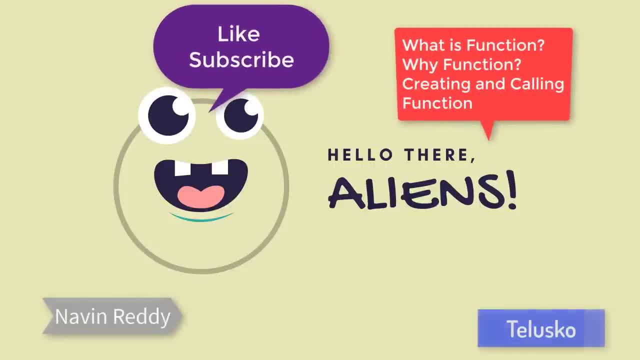 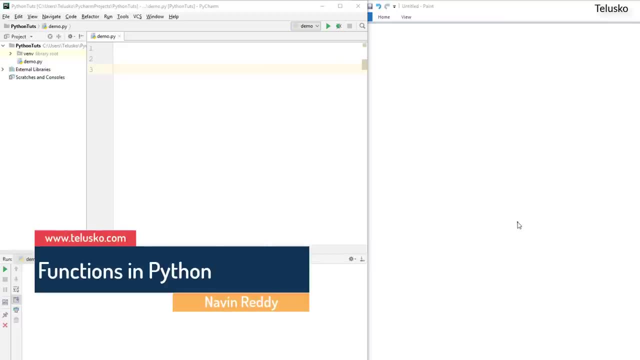 Welcome back, aliens. my name is Devyn Reddy, and let's continue with this series on Python Now. till this point, we have seen basic stuff, right, we have talked about variables, we have seen arrays, and then we have also talked about NumPy. Now, in this video, we'll talk. 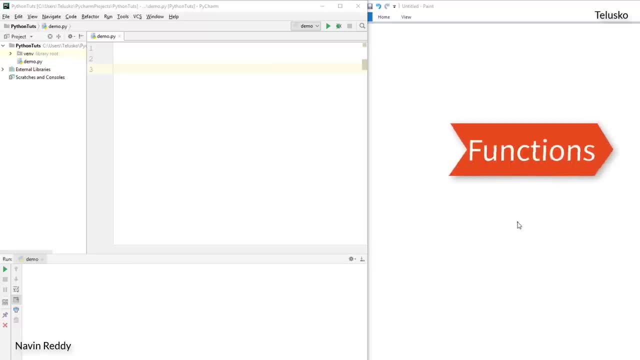 about functions, But why do we need functions? To understand this, let's take a scenario. Let's say you are working on a project and it might be a complex project or a simple project. Now, when you have a complex project, what you will be doing is you will be breaking. 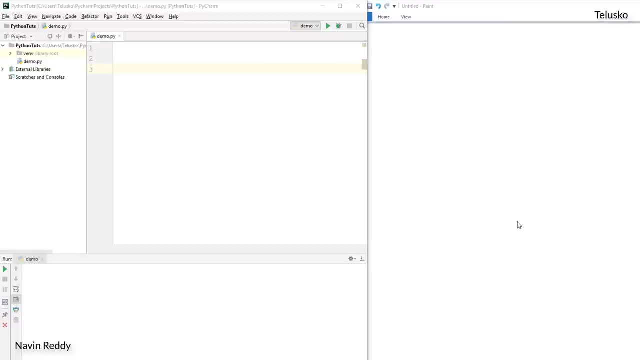 that project into smaller tasks. Now, when you talk about that small task, of course you will be writing multiple statements. For example, if you want to achieve, you want to perform a payment operation, Now in that payment you will be writing multiple statements. 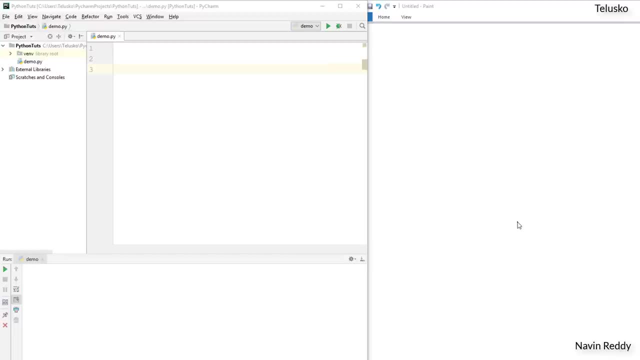 Now, all these statements you can keep it together so that you can reuse later. Example: let's say: if you have, there are multiple places where you will be doing the payment, So of course you will be using the same set of lines in multiple places. So let's say: 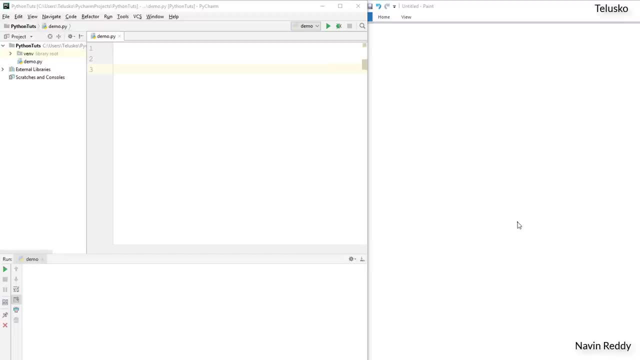 you have multiple places right So you can put them together, So you can imagine if you want to do any task. So make sure that all the statements of that one task stays together, And it should also be reusable, And that's where we will create functions. 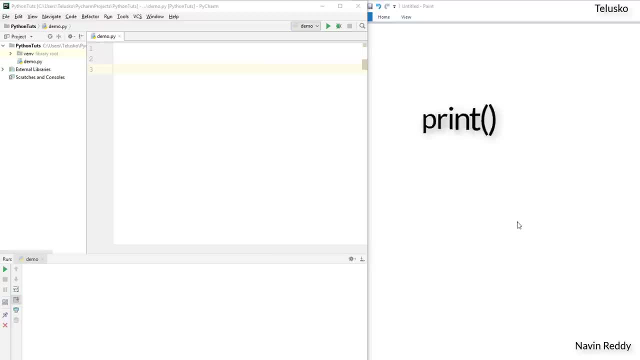 Now till this point. we have seen multiple functions- right. We have seen print. we have seen square root- right. We have used most of the inbuilt functions available in Python. Now can we create our own functions, Of course, right. That's what the video is all about. 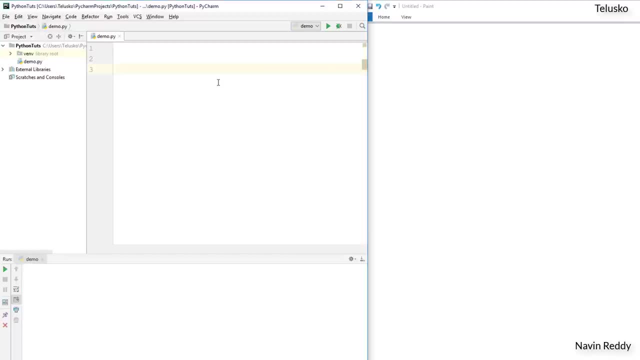 How do we create our own function? It's not that difficult. What do we do is so? there are two steps involved here. The first step is you will be defining a function, And second step is you will be calling a function. So let's go for the definition. 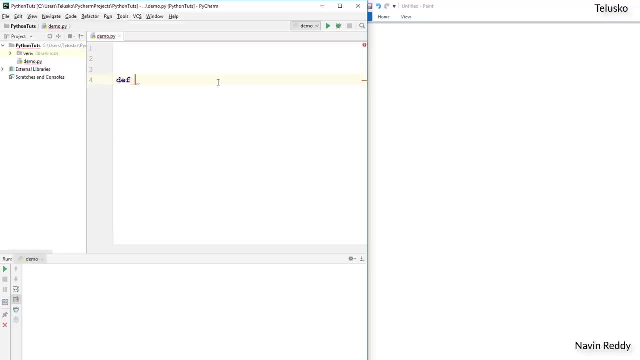 So you have to remember the syntax for it. Syntax is: you have to say def. that's how do you define a function. And of course you have to mention the function name as well. At this point I will say: greet, that's a function name. And whenever you work with 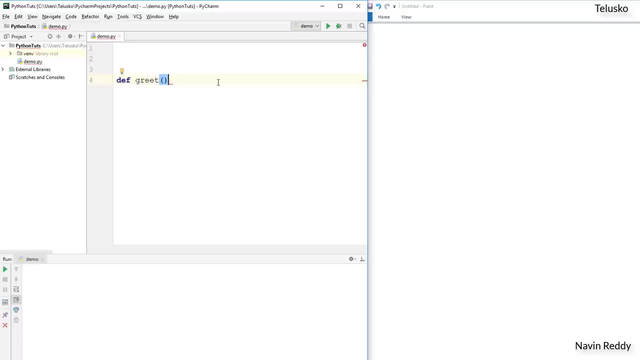 a function, you have to make sure that you put a round bracket here. So how do your? Python knows that It's a variable, it's a function, So you have to give a round brackets there. Now, once you define a function, you have to give a colon, because this function will have multiple. 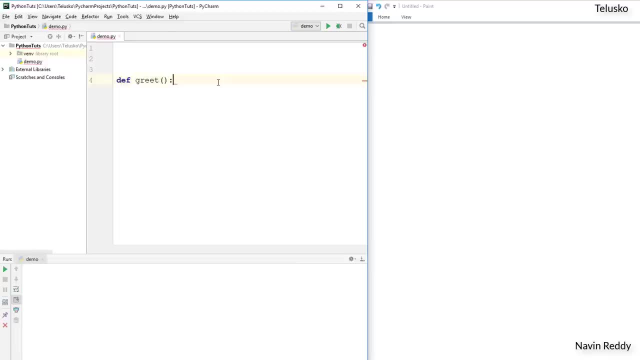 statements. right. Example: the same way we have done with for loop if else. right, Because in if or while you have, you might be having multiple statement. In the same way, in this function definition you may be having multiple statement. So you will say enter And this: 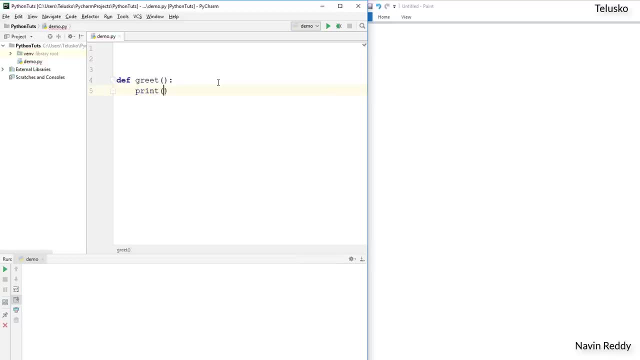 is where you will write your statements. I will say print. I want to print Hello, And then I also want to print good morning. So then I want to greet someone with this two things, which is hello and good morning. So what I'm doing is I'm putting those things in a function. Of course, you can do a lot. 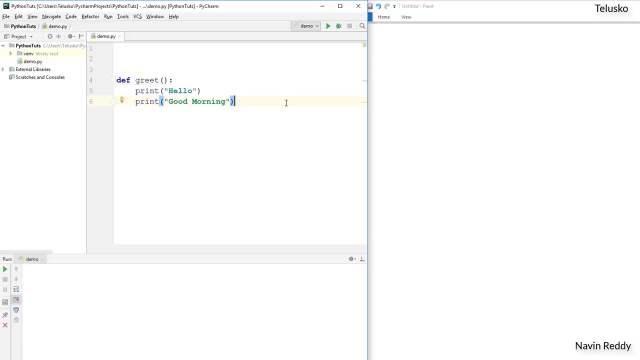 of big things in functions. Okay, this is just an example. So this is just your first step towards function. So let's keep it simple And later you can see what a function can do for you. So we got this function right Now. this is how you define a function. So step one is you have to. 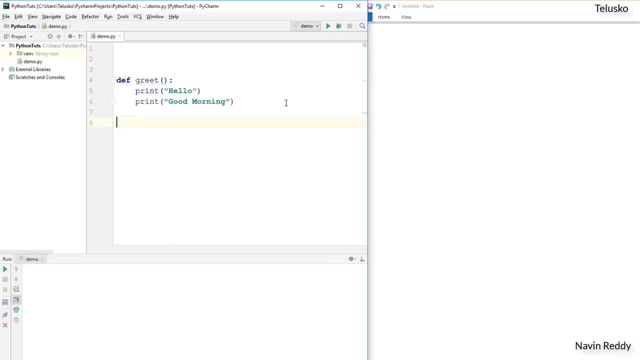 say def, and then you have to give a function name, then you have to mention a colon In that function, you have to define the statements, So this thing which are together, they are called as sweet. Now, once we got this, will it work? Let's run this code, Let's see what happens. 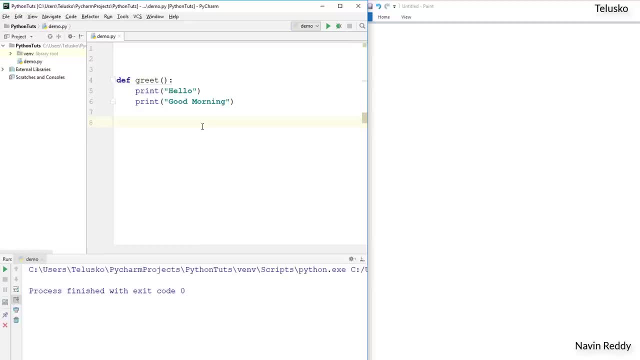 The moment you run this code you can see we got the output, but in output we are not getting hello or no, we are not even getting good morning. What's wrong? So the thing is, the function is ready for use. Okay, so we have defined the function, So this function will be called only. 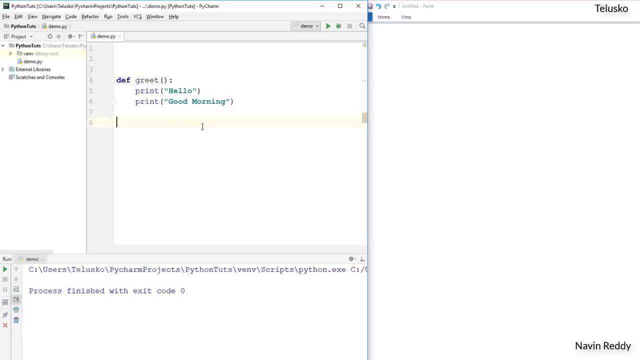 when you are explicitly calling it. Of course you have to call it right. How do we call that? the way We call other functions right? When you work with print, when we work with square root, we just have to call it right. So you have to say great bracket, right. So this is your. 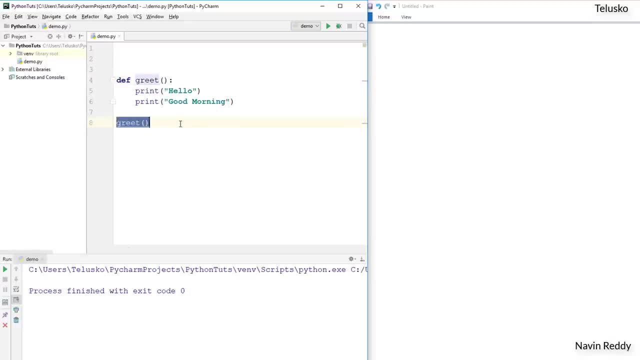 function definition. So this is your function definition And this is your calling. So if you don't call, it will not execute the function. So if we run this code and you can see, we got the output, This is how you define a function. a beauty right Now, of course, as I mentioned, 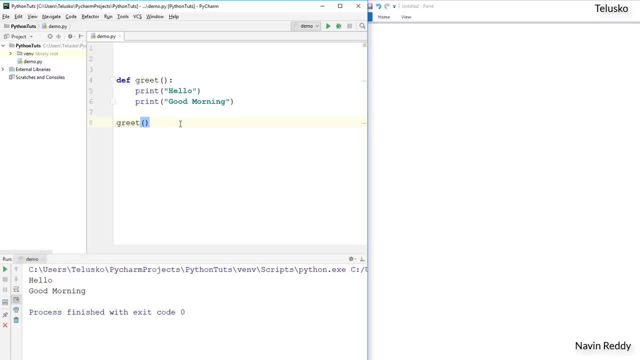 using function you can do a lot of stuff right. You can ask a function to do something for you, Or you can imagine in your project your one function is your one helper. So let's say, if you're building something big, you need 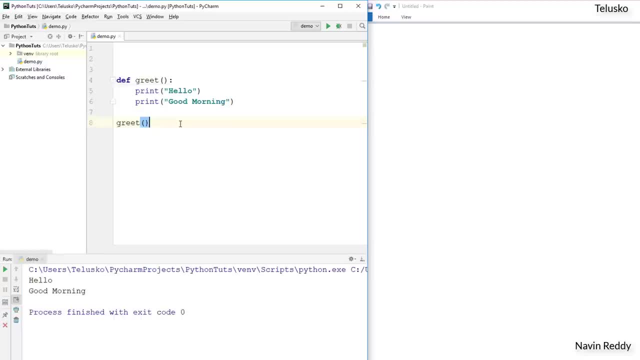 some help, right? So you can say, hey function, this is your job, Hey, other function, this is your job. You know in the industry the way we allocate project to everyone or allocate the task to every person. In the same way you can allocate your task to every function. Of course you have. 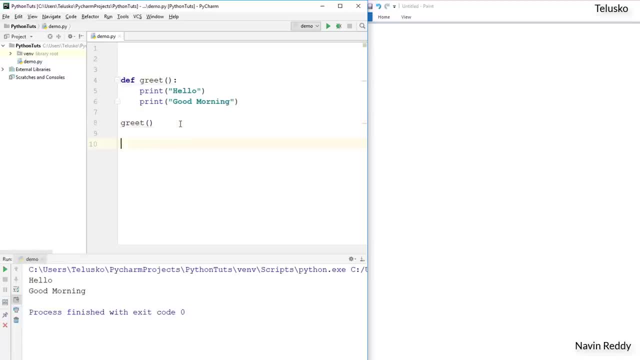 to define the function as well. Now you can call this function multiple times. So let's say, if you have a big project of 1000 lines, and in that this is the fifth statement, And after, after some statement, I want again, I want to greet, So I will say greet. 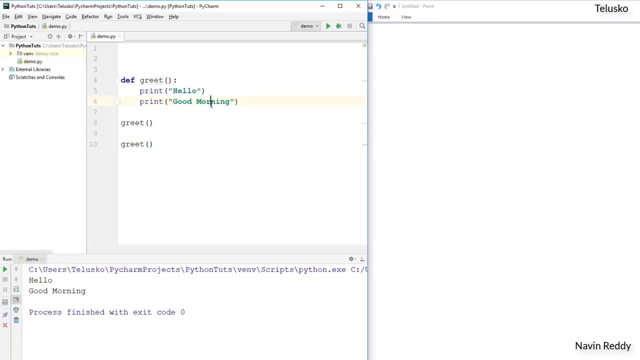 You don't have to repeat those statement. you don't have to say hello, good morning every time. just define it once And you can call it multiple times. right, Let's run this code And you can see we got Hello, good morning two times. That's, that is what we want, right? Okay, now let's do. 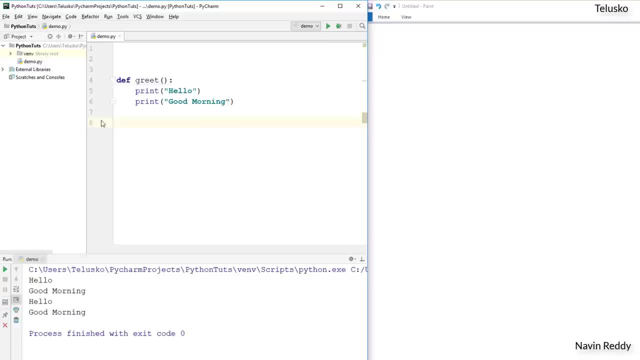 something different. Of course, we'll be working with functions. What I'm going to do is: I want to add two numbers. you know the simplest example of functions, right? So let's go for addition of two numbers. How will you add two numbers? I want to say, hey, I want to add because, see till this. 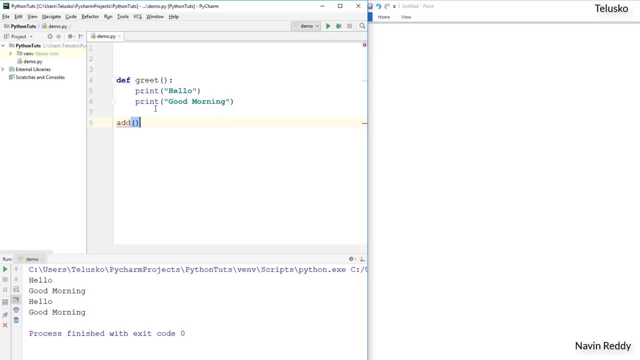 point. we have seen multiple functions, right, We have seen square root, we have seen power. But then those functions are inbuilt And of course we have to pass parameters as well. So when I say parameters, the variable, the data which you want to perform, example, when you say square root, in the bracket, 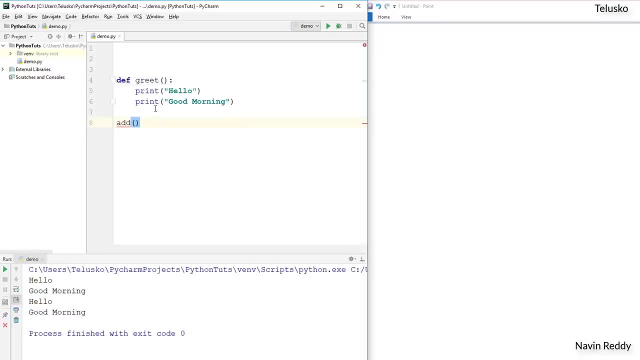 you mentioned for what value you want a square root of. So here as well, in this ad, you have to pass a value. I will say, hey, I want to add four and five. I don't know the output, I just want to. 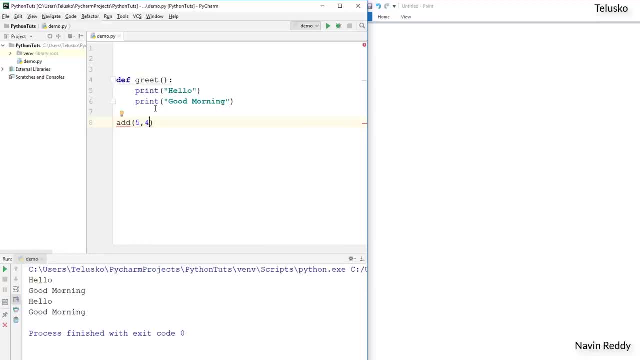 add these two numbers. But the question is: do we have this function available? Of course not right So way to define one more function. Now, this is a different function here, So we'll say def And we have to, so we have. 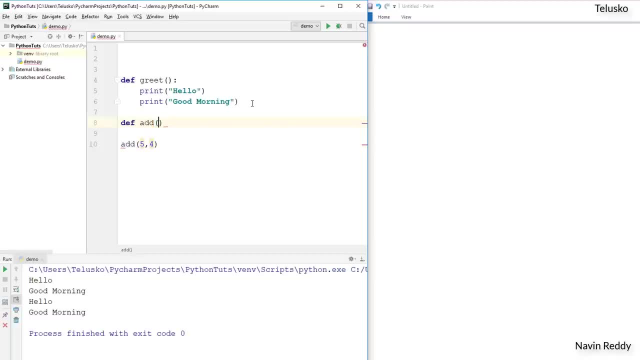 to mention a function name which is add. Now this function will take two parameters. Okay, now this is important. Okay, remember this keyword called parameters, or you can say arguments, So normally we can call them as arguments. So we'll say we have to pass two arguments here. One is x and y, So 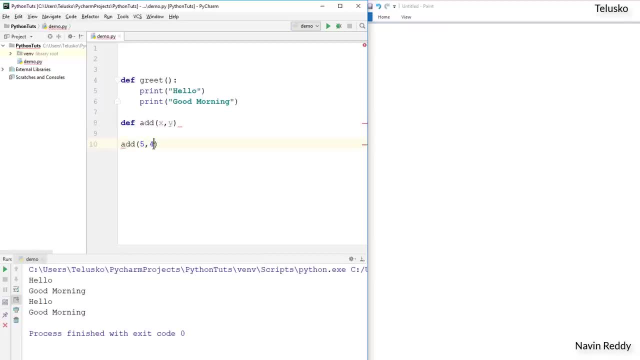 what are value you're passing from here, which is, you're seeing, add five comma four. you have to accept it somewhere, right? So you have to say x which will have five, You have y which will have four, then to give a colon, not so far. And here you can perform your. 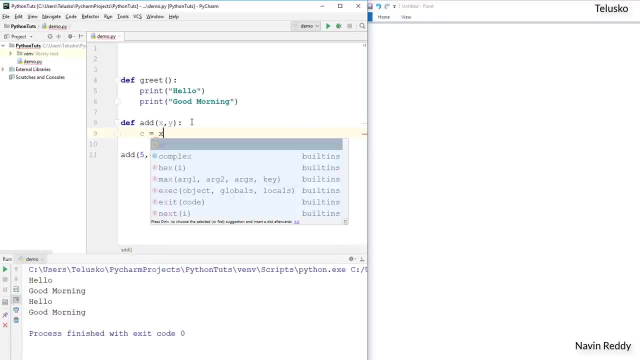 operation. So I want to say C is equal to x plus y. that's how you add two values right or two numbers. Now, once you have done the addition, you will simply print it. Now the advantage is: next time when you want to add two numbers, you don't have to say c equal to x plus y, you don't have. 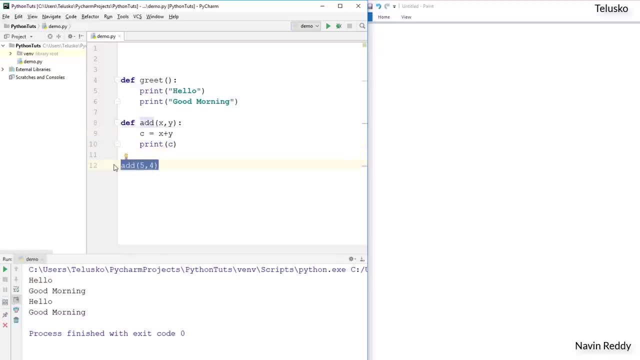 to perform this operation, you just have to call this function, called as add, by passing the values it will add for you. Now, if you're focusing on simple stuff- normally when you work on a project you do complex tasks with one function- Let's run this code, let's verify if it is working And you can see we got. 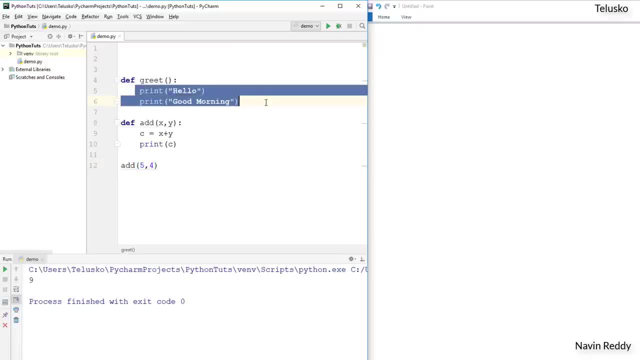 nine. So yes, it is working. Now you can see we have. we have not got Hello good morning. because we have, we are not calling great right? So if you want that output as well, we need to call them. So important thing is you can create multiple functions and you can call them as many times as 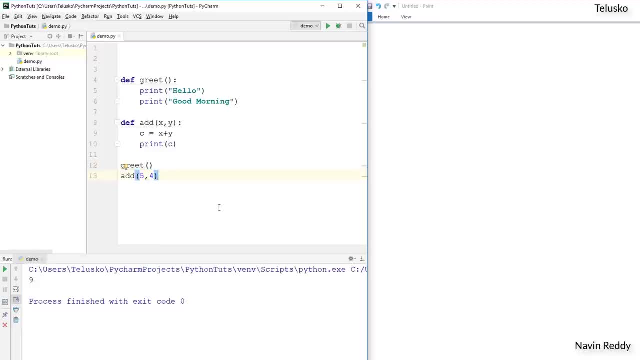 you want. So this is fun, right, But there's one more thing you can do. See, as a function you have one when you, when you call a function, a function, will do a task for you, So that the function which 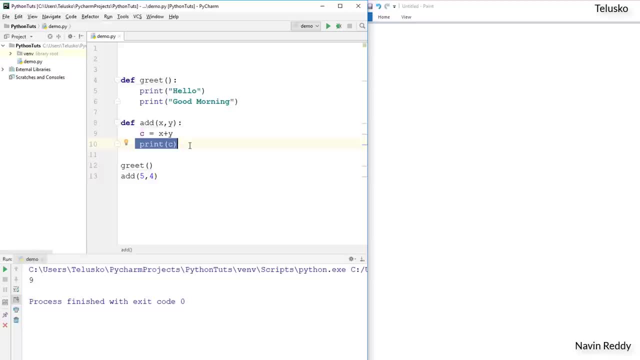 is you are using here is pretty simply printing it, right? Then we have another type of functions which will return you the value example. let's say I don't want to actually print it, print the value, I just want this addition of to these two numbers, and then I want to save it in some value. 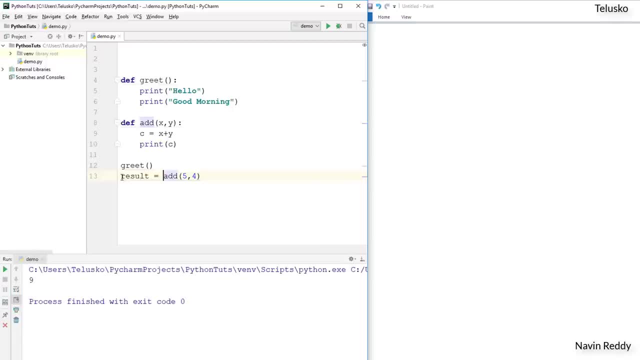 I would say result Example when you work with square root. remember when we worked with math module and then we had square root. the square root function was giving you something right, So your function can return a value as well. To understand the scenario, let me just take an 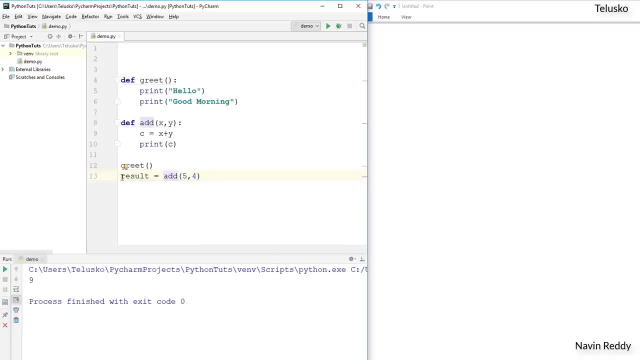 example here. So let's say if you are watching this video, and so let's say if your name is Rahul. so I will say, Hey, Raul, call Tina and say tomorrow I will be late for the session, So I'm. 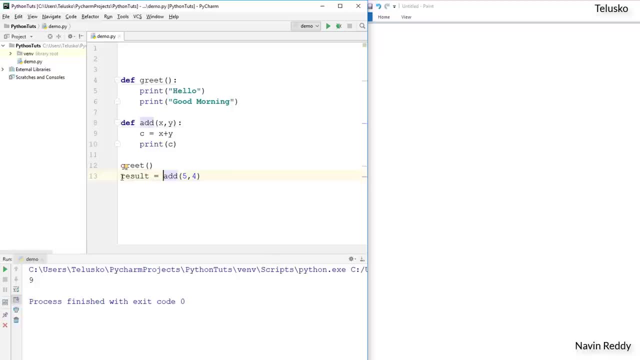 not expecting anything in return. right, That's one scenario. The second scenario is I will say: Hey, Raul, ask Tina what time. we have a session tomorrow. So this is where Raul, as a function, will return me something. So function can be of two types. a function will execute the task. 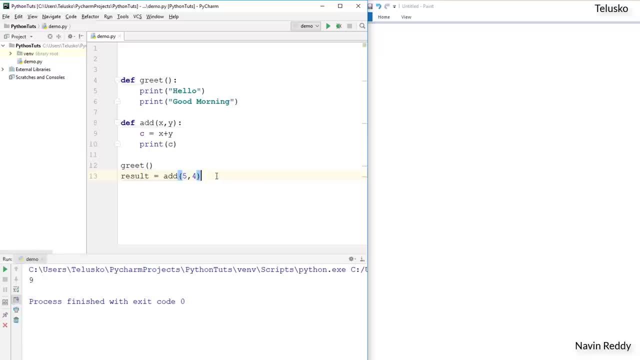 or a function will return you something, right. So in this, in this scenario, I'm expecting something. So when you define a function which will return something, you have to do that. you have to say, instead of printing it here because I don't want to print, I will say return. 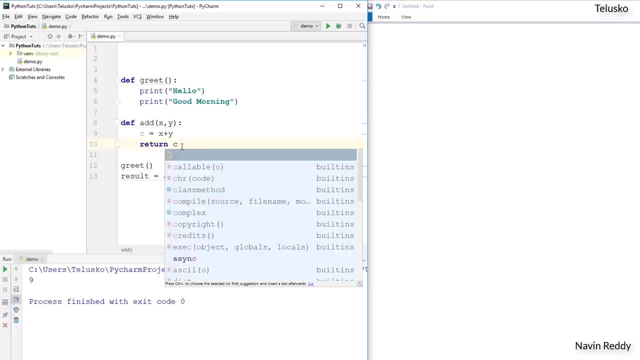 and they have to return C. So return is a keyword which we use to return the value. So what you're doing is you're saying, Hey, add function, add these two values and give me the addition. Okay, so whatever the addition is, it will be assigned to this result. Now it is your choice, if you want. 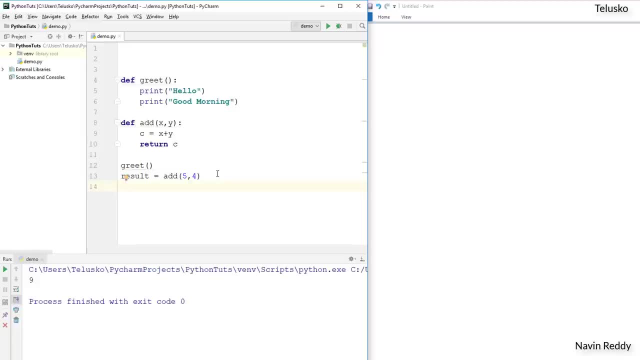 to do this. if you want to print result, if you want to store you this result into database, or you want to post this result on Facebook, I don't care. what I care is: I am giving you the value. I'm not responsible to print it. I'm not responsible to put that value on Facebook. 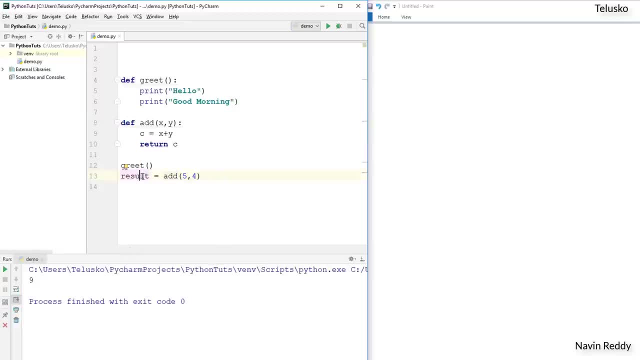 I'm responsible just to add those two values. you can do whatever you want, But then here I just want to print it because I don't want to write a code for Facebook here. So I will say result And let's run this code And you can see we got the output. So this is important. 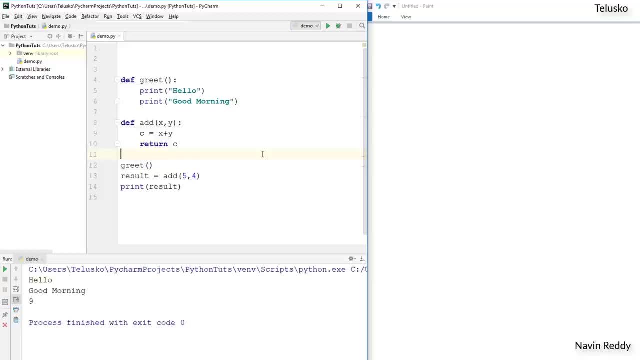 a function can return a value of function. you can write a function which will not return a value. Okay, this makes sense right Now, time being, just to make it clean. I will not be using this with a great thing. So these are. we can define a function. What if I? 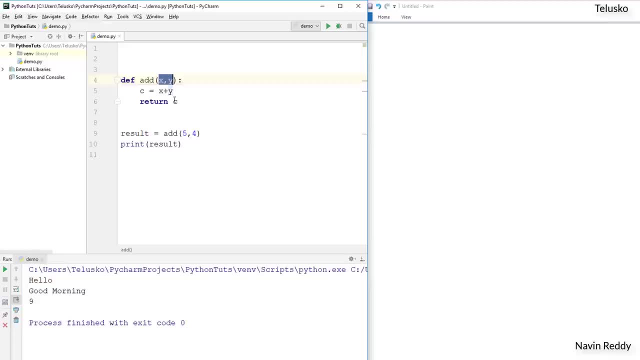 want to return two values, Because, see, we are passing two values right And we are returning only one value. What if I want to return two values? but what do I use our return? let me just change this to have another main name called as add and sub, So the function name itself. 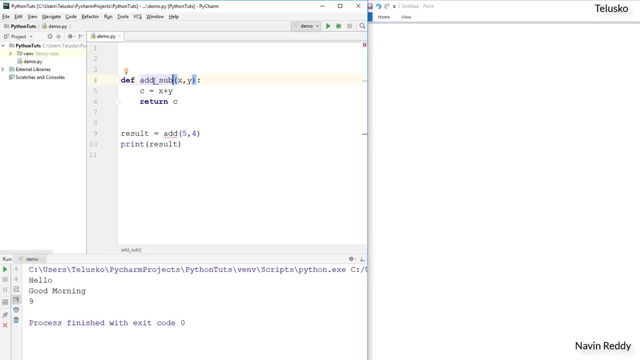 is add, sub, And you can guess it now. this will provide you two things: the addition and sub fraction as well. So let me take two variables here. one is C and one is D, and D will take x minus y. So in total we have two results here, C and D. I want to return both, So I will say C comma D. 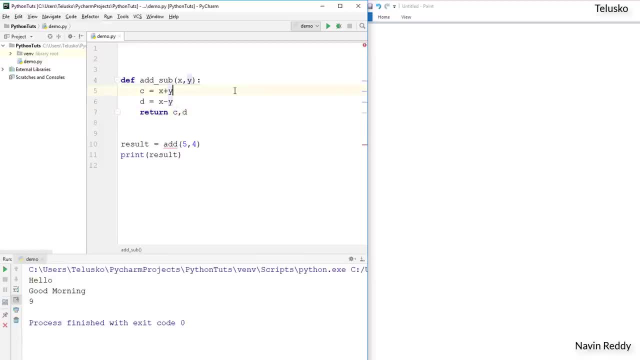 So yes. so yes, you can return two values, Okay. So you can call a function. a function will accept two values or multiple values, your choice, and you can return multiple values, Okay. but there's one problem. you can see we are getting error here. it says unresolved. So we'll say: hey, function.